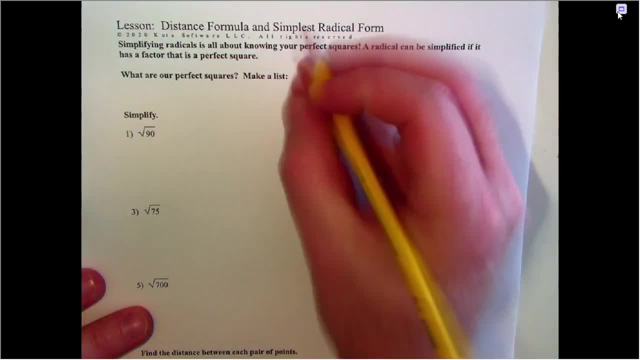 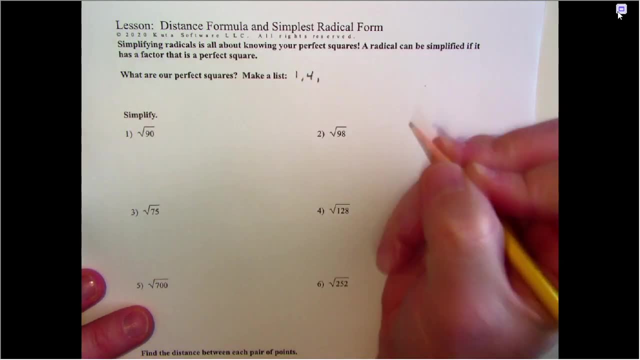 So it's all about knowing what are your perfect squares. You might want to make a list, All right. so 1 is the first perfect square, 4 is the second perfect square. 9,, 16,, 25,, 36.. 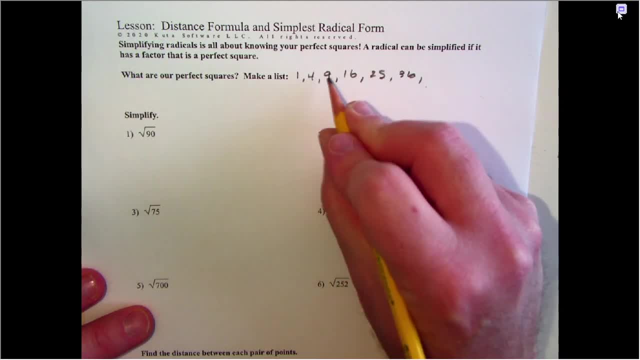 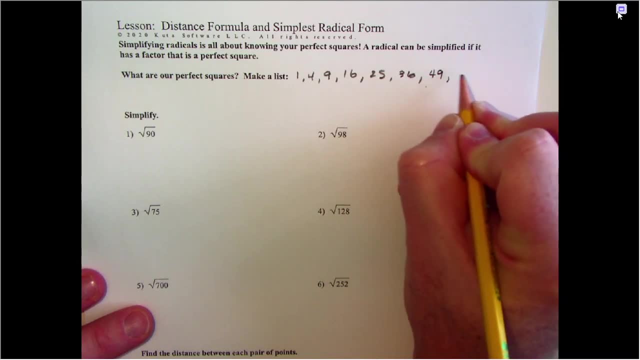 If you don't know where I'm getting these numbers, it's just 1 squared, 2 squared, 3 squared, and so on. So I'm up to 6 squared is 36,, 7 squared is 49, and 8 squared is 64.. I'm not sure why. 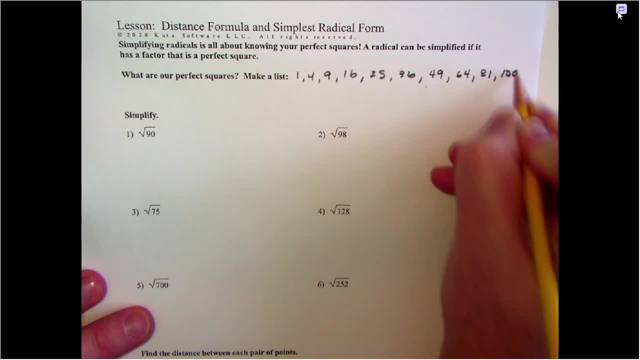 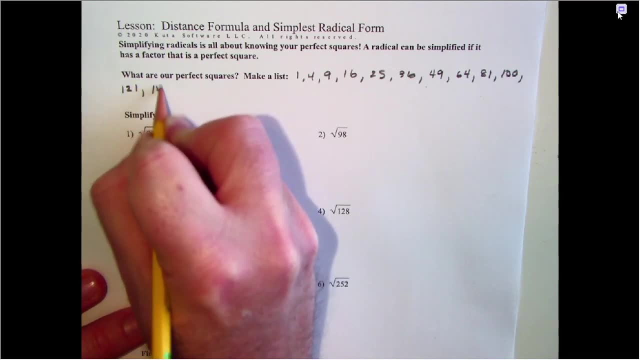 I had to think so long there. Then 81, then 100.. You know, I'm going to continue this list a little bit here. 11 squared is 121,. 12 squared is 144.. Typically, if you at least know, 1 through 10,. 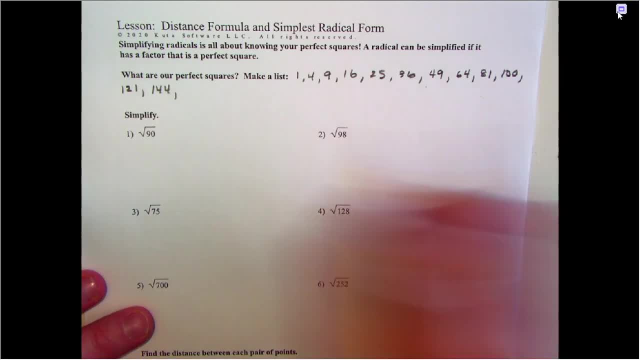 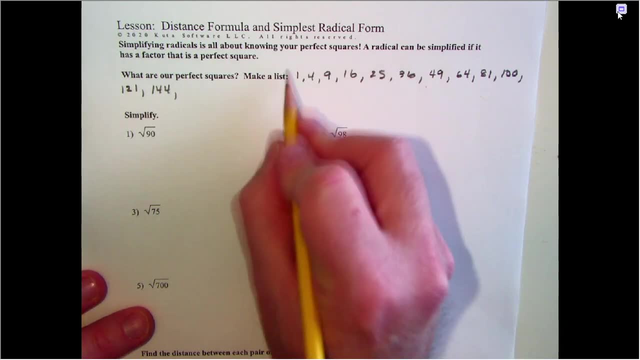 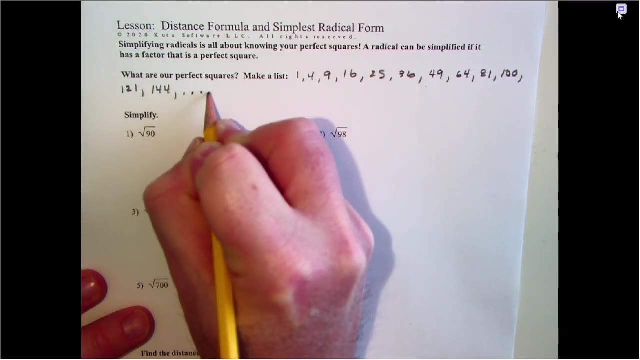 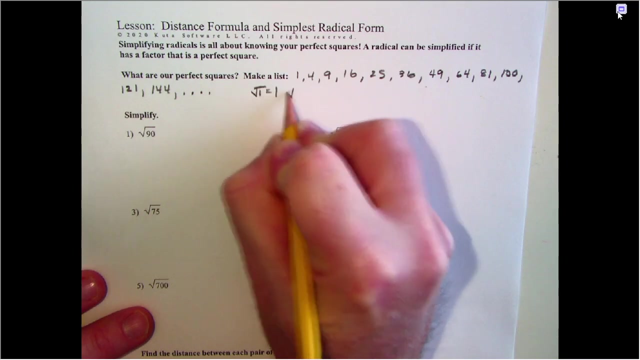 that's good, All right. so perfect squares. what that means is these have a perfect square root, Like if I took the square root of all these numbers, the square root, and again I could keep going past 12 if I wanted to. The square root of 1 is 1.. The square root of 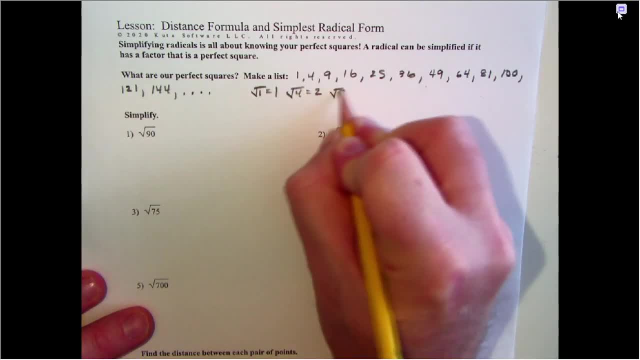 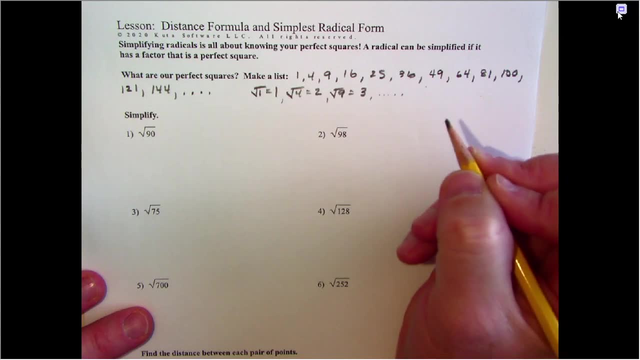 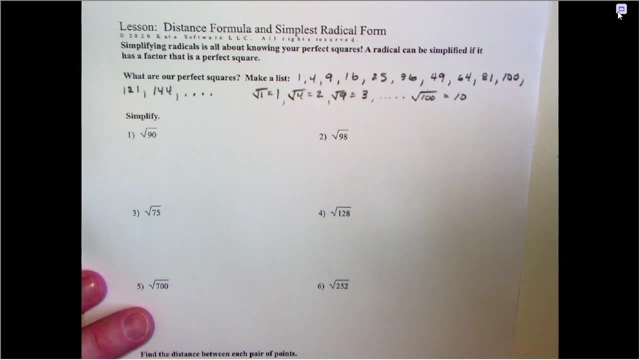 4 is 2.. The square root of 9 is 3, and I could go on and on. These are all perfect because their square roots are nice whole numbers. All right, the square root of 100 is 10.. That's why they're called perfect squares. 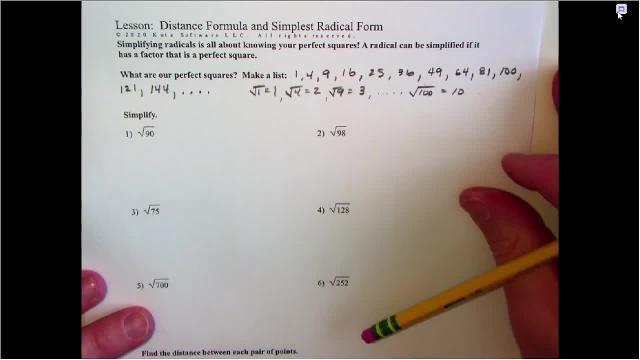 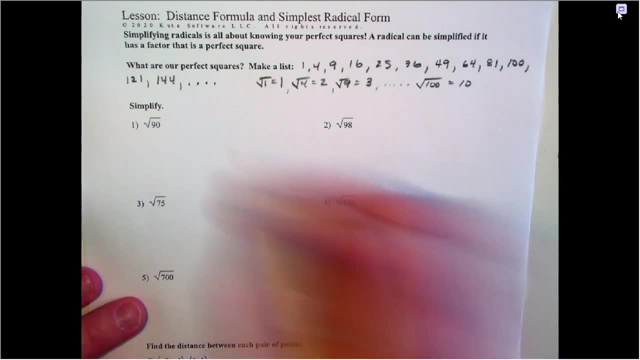 What I have here is some examples of non-perfect squares. I'm not going to do all of these in this video lesson, but I'm going to do some of them because the process is very similar. So it's all about breaking down these numbers into their factors. Now, 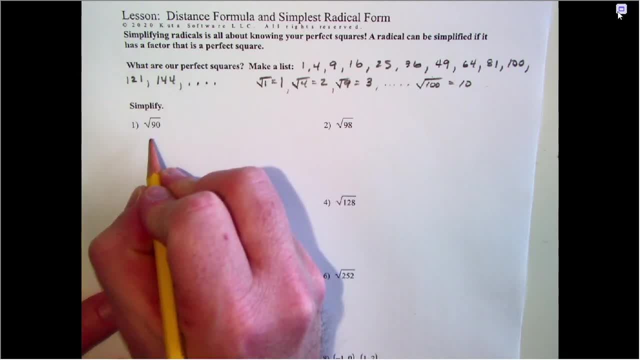 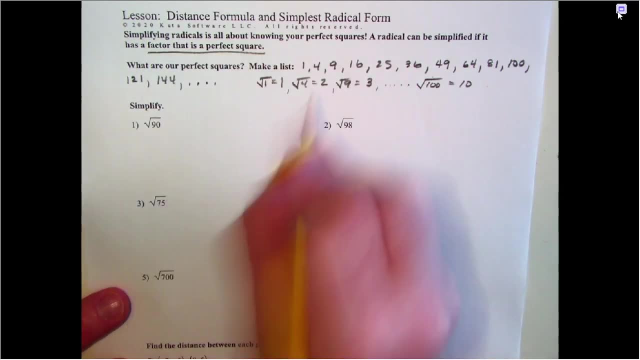 we don't want to just look for any factors. We want to look for factors that are perfect squares. Now, if 90 doesn't have any of these numbers that are factors of it, then it can't be simplified. So there are some numbers that cannot be simplified. 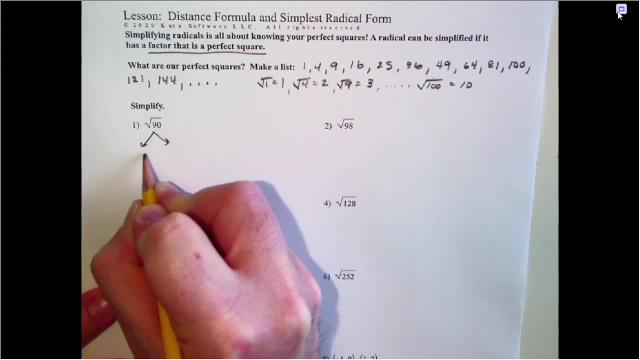 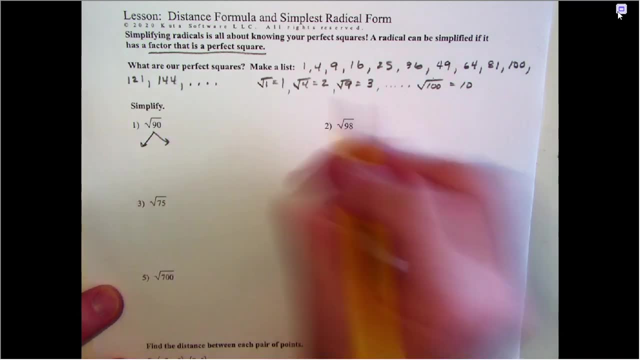 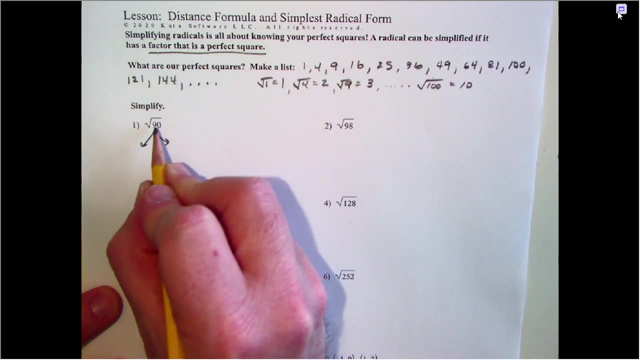 So the square root of 90, I'm going to break it down into its factors. Now, I'm not going to choose 45 and 2, because 45 is not a perfect square and 2 is not a perfect square. So we want to look for perfect square factors that go into 90, and the trick is we want to pick the biggest. 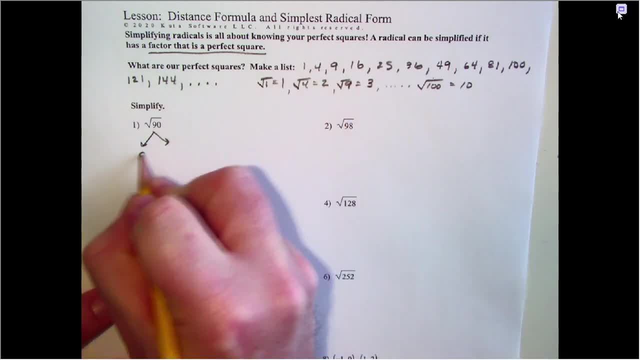 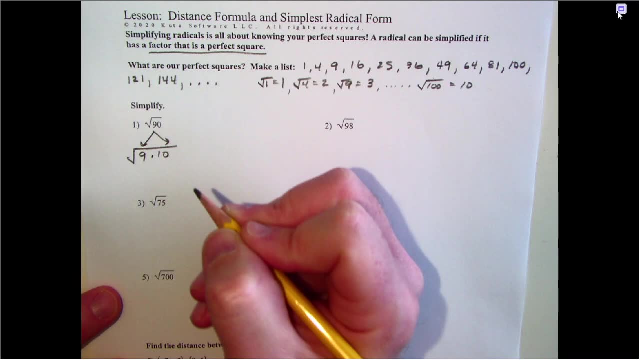 Well, I know our way. 9 goes into 90 ten times, so I'm going to write this as the square root of 9 times 10.. Now, you might have done a little bit of this in middle school math- Great. 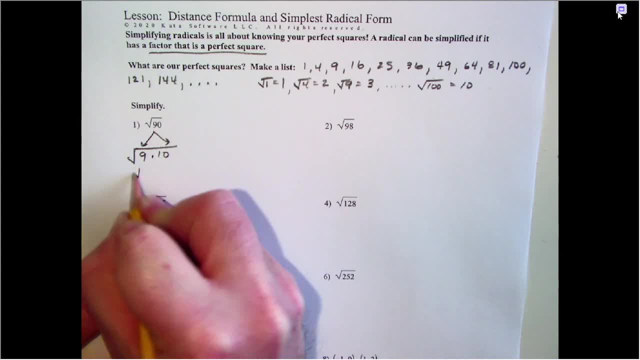 So I can break this down now into the square root of 9 times the square root of 10.. Now I'm going to go up here and look 9's on my list, which means it's perfect, which means it has a perfect square root. So the square root of 9 is 3.. 10 is not on my list here. 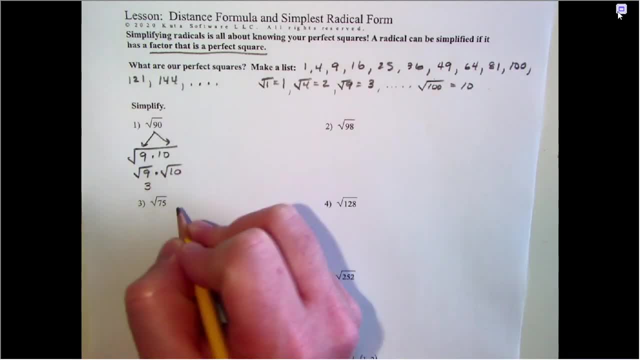 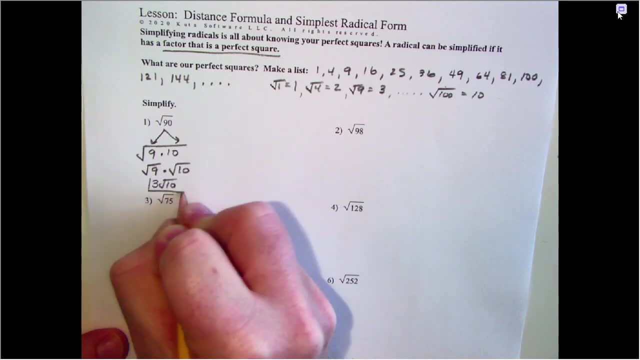 The square root of 100 is 10,, but that doesn't say the square root of 100 is a square root of 10.. So here's what happens to the non-perfect square: The non-perfect square stays underneath the radical and we end up with an answer of 3. 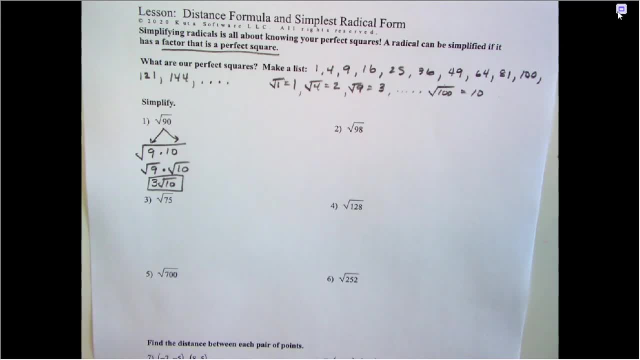 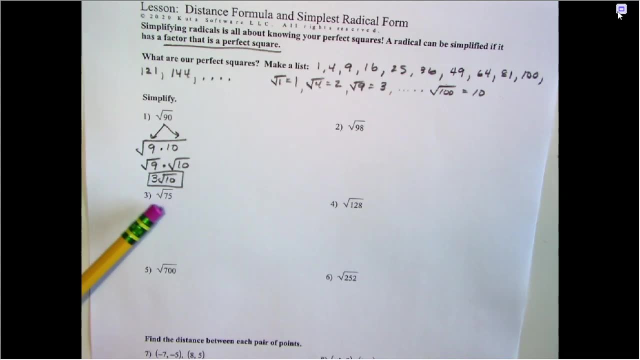 square roots of 10.. All right, This one's probably pretty obvious to some of you that you know what 25 goes into that 3 times. So I could change this to 25 times 3.. The better you get at this, the less. 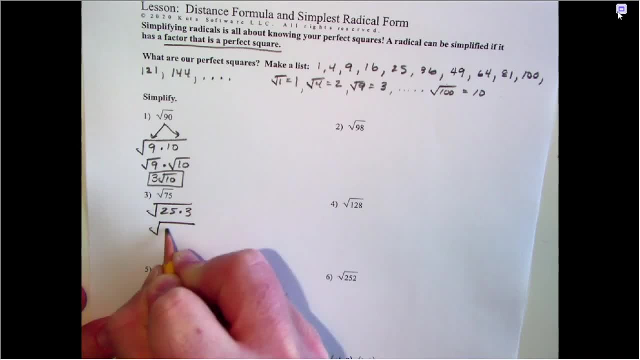 breaking down you're going to have to do. If it helps you to break this down to square root of 25 times the square root of 3, do that. Square root of 25 is 5.. Square root of 3 stays square root of 3.. 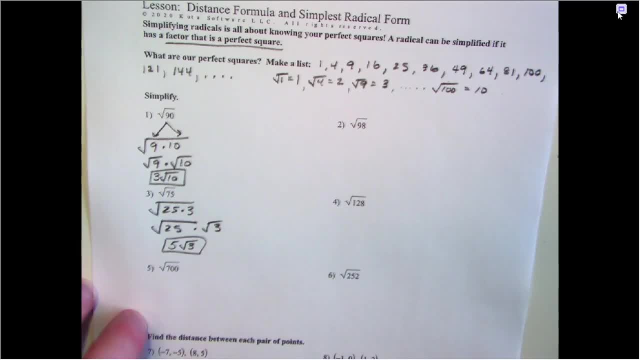 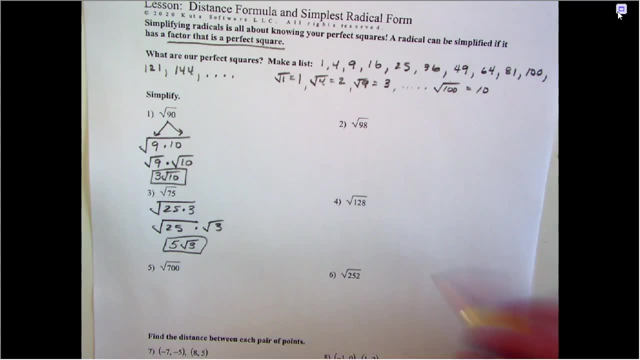 All right, let's do one more here. Let's do 252.. Let's break that guy down. Well, 252, that's a pretty big number. I don't know off the top of my head which one of these goes in there. So you know what? I'm going to grab my calculator for a little support. 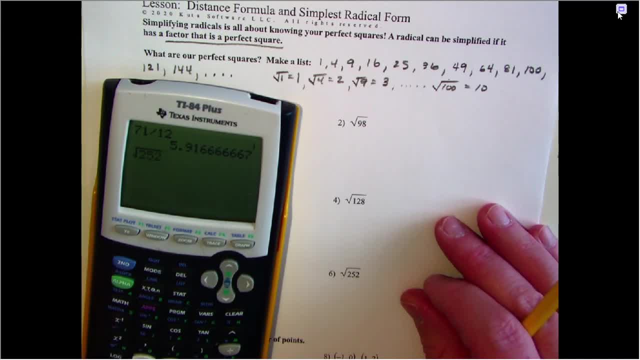 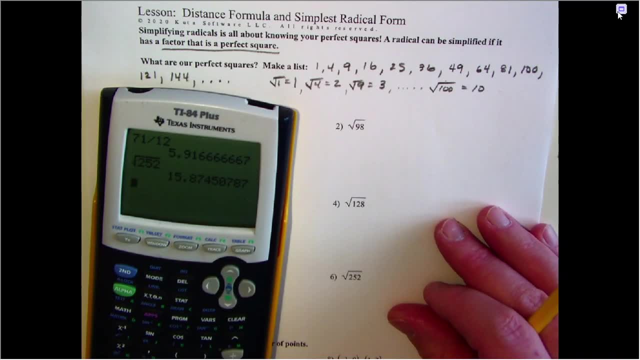 What your calculator will not do for you is simplify our radicals. You know I could tell you what the radical is as a decimal all day long. Now, in Lesson 1 of this new module, you guys could have given me the distance in decimal form. That'd be fine If you already knew how to do radical form- great. 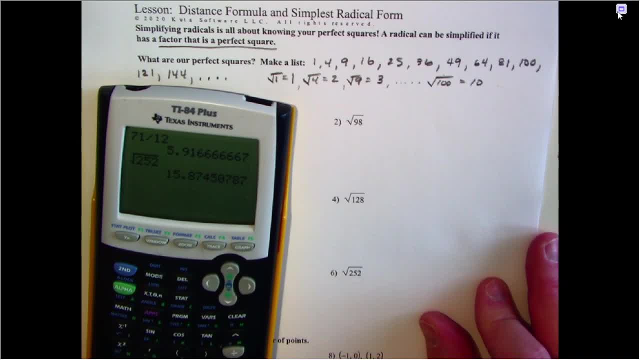 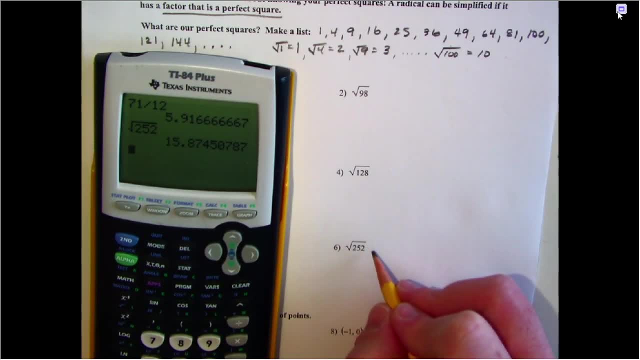 From this point forward, we're going to try to do exact answers. We're in simplest, radical form, as much as possible. All right, so let me demonstrate this real quick: 252, so I know 25 won't go in there, Let's try 16.. 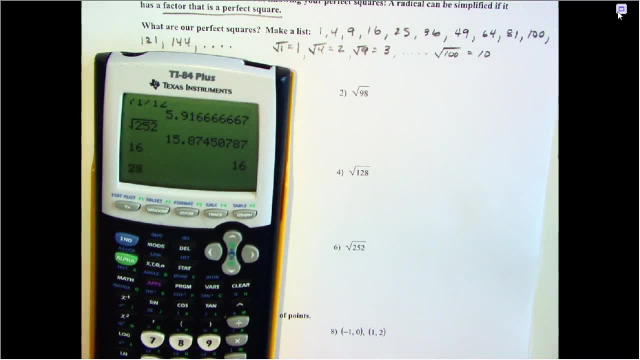 Does 16 go into 252?? Well, I got to type in 252 and divide by 16.. No, it doesn't go into an even list, so it's not a factor of it. Let's try 252 and divide it by 36.. Oh, it does. 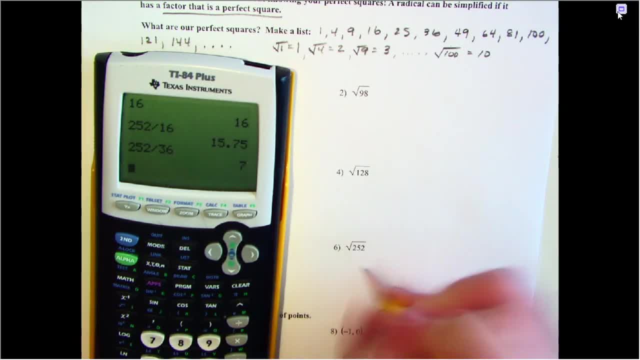 7 times- And I know that's probably the answer- because 7 is a prime factor And prime numbers are not divisible or can't be broken down anymore. Now this might be a classic example where some of you might have tried 4.. 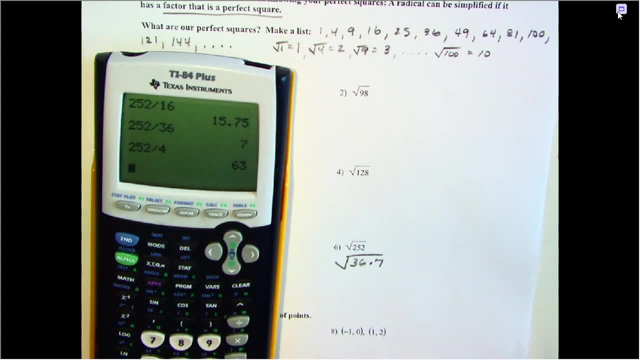 Hey, 4 does go into it, But if you used 4, you're going to kind of get trapped there If you said that's 4 times the square root of 63, so you're going to write this answer for me. 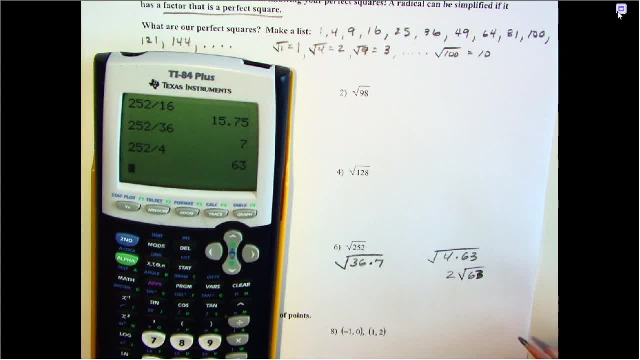 4. Sorry, you're going to write It as 2 square roots of 63. But 63 still can be simplified. So kind of the trick here is we want to pick the biggest perfect square that goes into these numbers. So you might have to use a calculator to start doing some dividing. 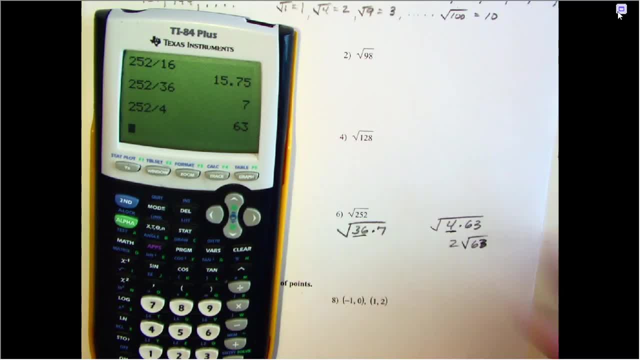 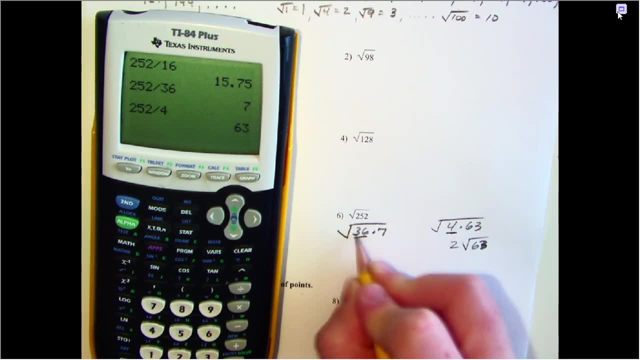 If you don't know your factors off the top of your head, I don't know who knows their factors of 252 off the top of their head. So grab a calculator for a little support. So here's my perfect square. The square root of 36 is 6.. 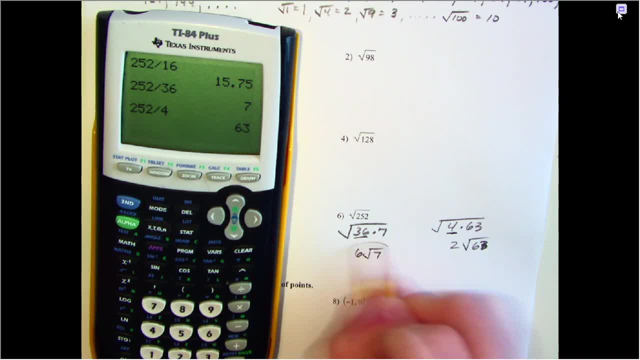 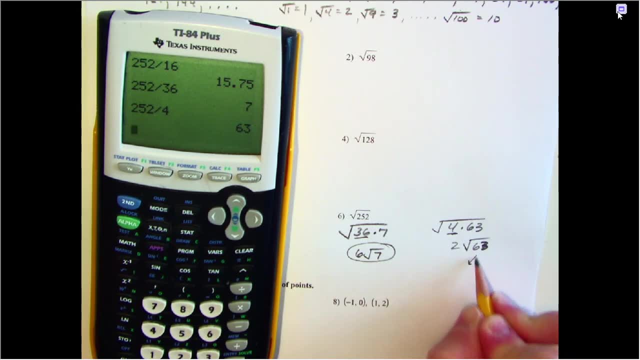 It's not a perfect square. It stays underneath the radical. If you chose this, you could still get to the correct answer. You're going to have to break down that 63.. So this would be 2 times the square root of 9 times 7.. 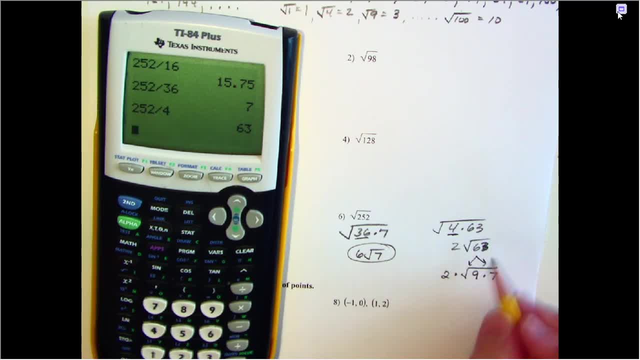 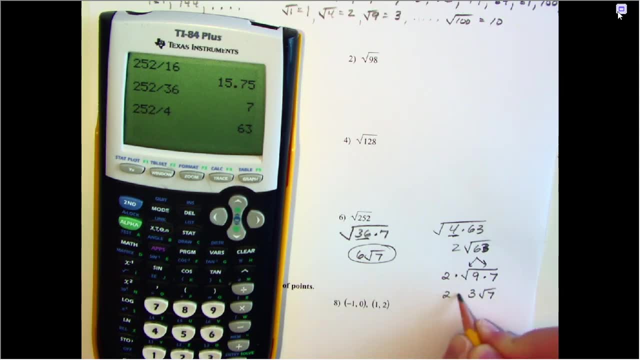 63.. I hope everybody knows 9 times 7 is 63.. 9 is one of my perfect squares, So guess what? I could take the square root of it And the 7 stays under there, But I got this 2 out here. 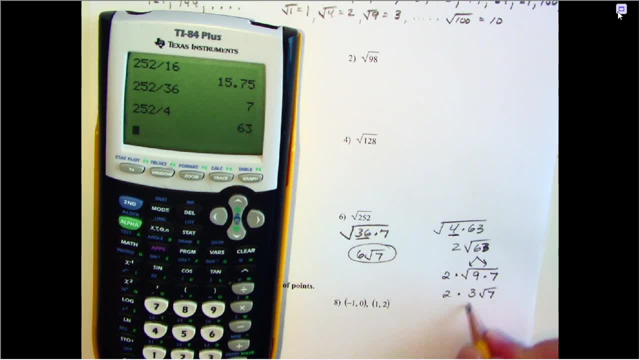 I got this square root. The square root is the same number as the 2 in the front. You have to do an extra step if you chose 4.. You will get the right answer if you don't choose the biggest one. You have to keep simplifying. 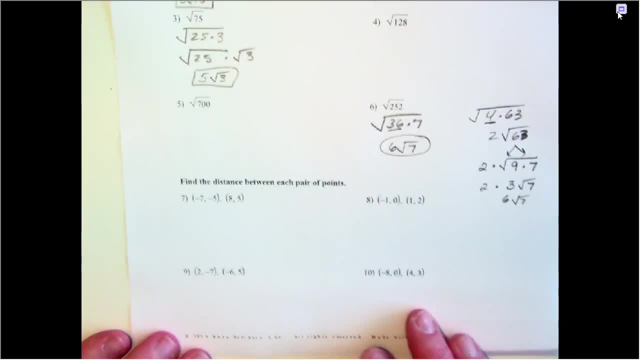 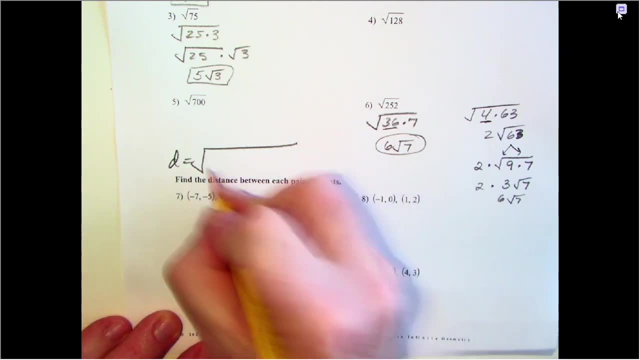 Let's demonstrate this using the distance formula. In the previous lesson, we learned that the distance formula is the square root of x2 minus x1 squared, plus y2 minus y1 squared. All right, So you've had a little practice on this already, but you were not required to put it in simplest. 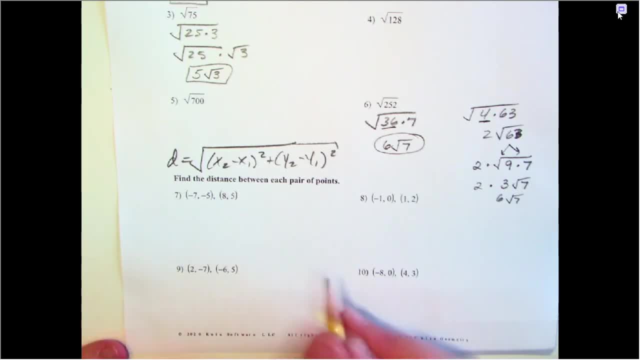 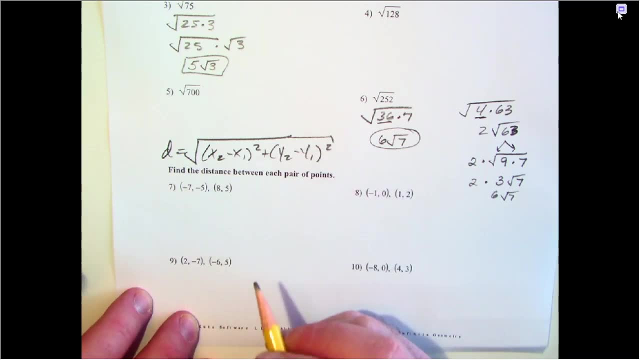 radical form. We're going to do that in this particular activity or assignment. Don't be surprised if, going forward, it asks for everything in simplest radical form. I like simplest radical form because it's exact. All right, let's do one or two of these here. Let's just do number. 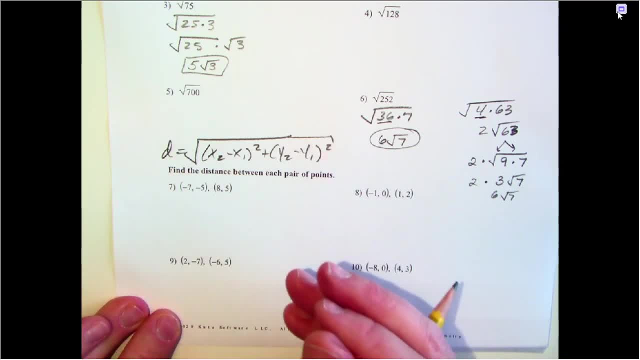 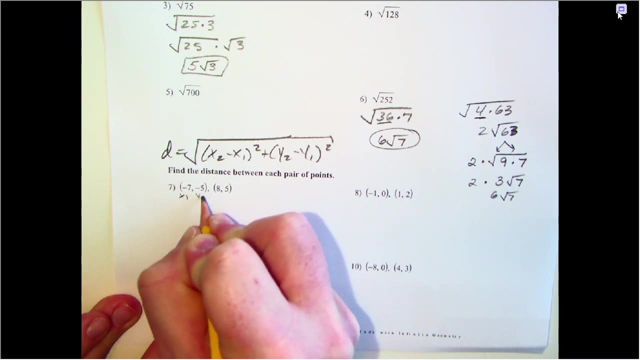 seven here. By the way, I can post this on Canvas as well if you want me to this document. If not, just shoot a note, but paper will be sufficient, All right. so let's see: That's x1,, that's y1, that's x2,, that's y2.. I like to label those All right. so my distance. 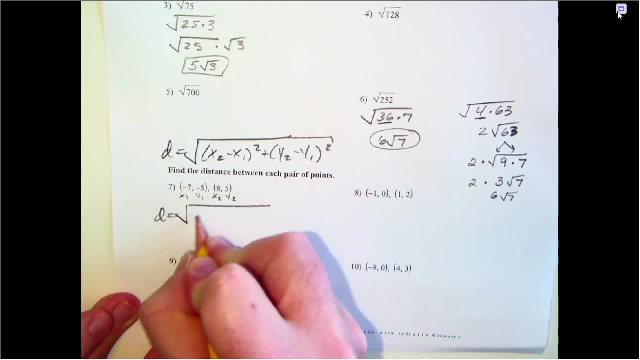 is going to be the square root of 8 minus a negative 7 squared, Plus 5 minus a negative 5 squared. All right, and I'm going to take care of these minuses. So I know this is 15 squared plus 10 squared, and all that's still underneath the square root. 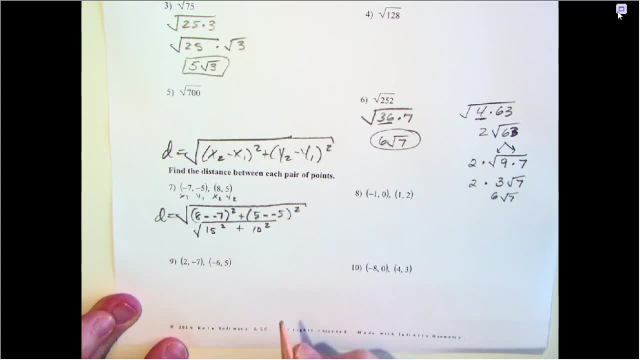 I hope you don't have to change that to a plus. You can do that in your head. Well, I know 15 squared is 225, and I know 10 squared is 100. If you need help with a calculator, there is no shame in that. 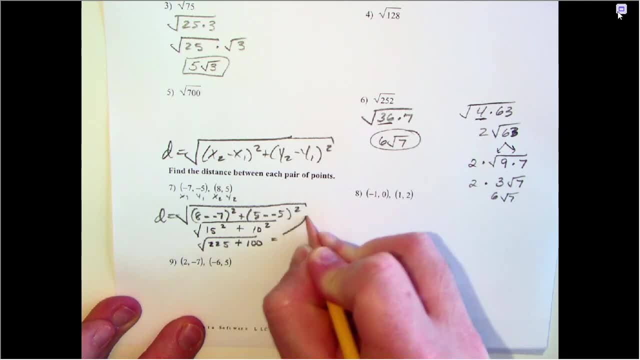 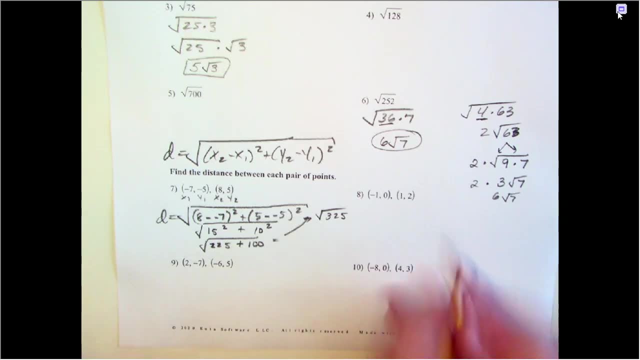 So this comes out to the square root of 325.. Now that is not in simplest form, So I get to put it in simplest form. I hope this 25 is kind of a red flag here. Hey, 25 is on my list of perfect squares up here. I bet it goes into it. 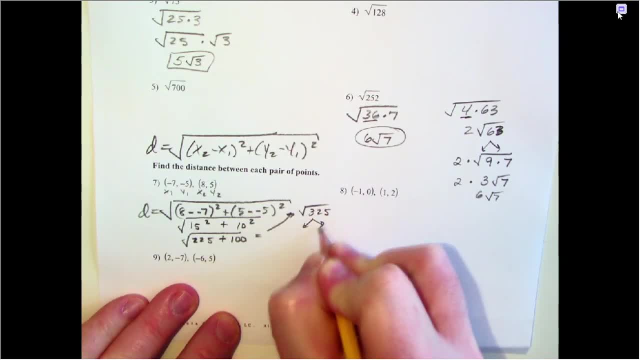 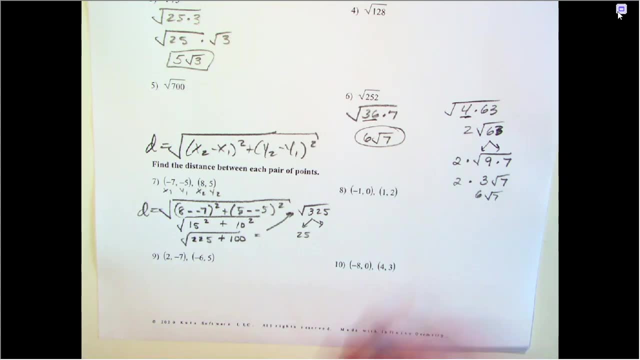 So I'm going to break this down into 25 times something. If you need a calculator, take 325,, divide by 25, and get 13.. So this is the same thing as the square root of 25 times 13.. 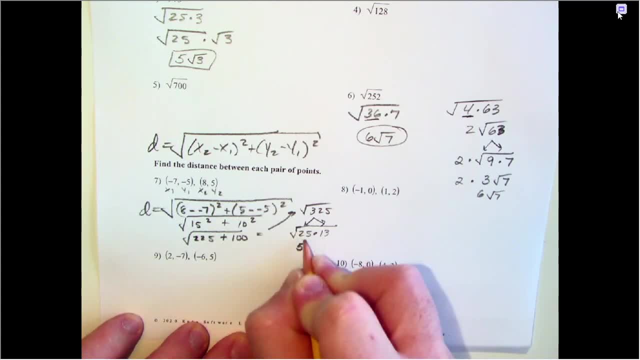 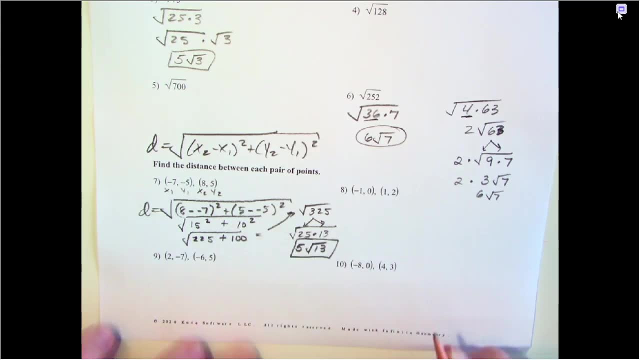 Well, the square root of 25 is 5.. That comes out of the radical. The 13 is not perfect, It stays underneath the radical. So my distance is 5 square root of 13.. What I do not want you to do here: if the directions say: 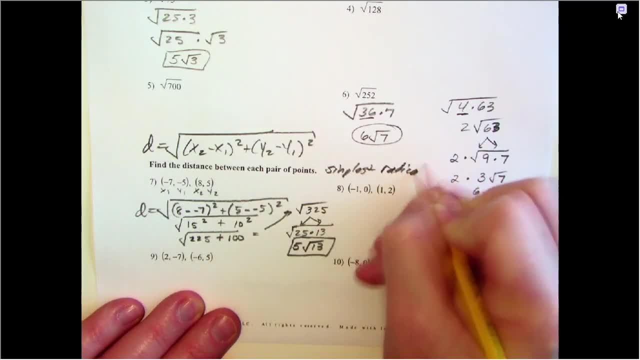 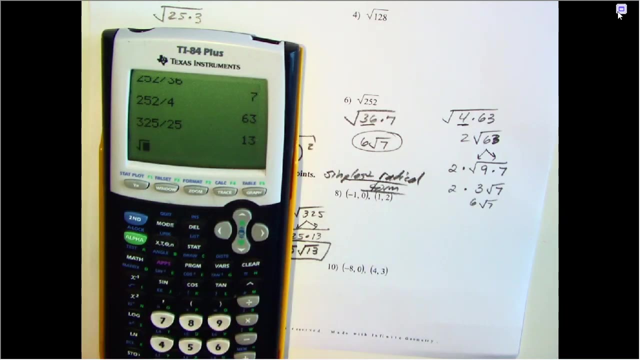 simplest radical form. I expect to see this work and I expect to see you simplify the radical. If it says simplest radical form, it doesn't. You can give me a decimal answer, but what I don't want is this: I will count it wrong if you type in and give me. 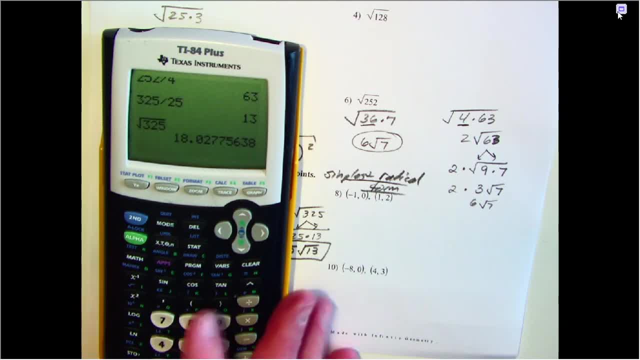 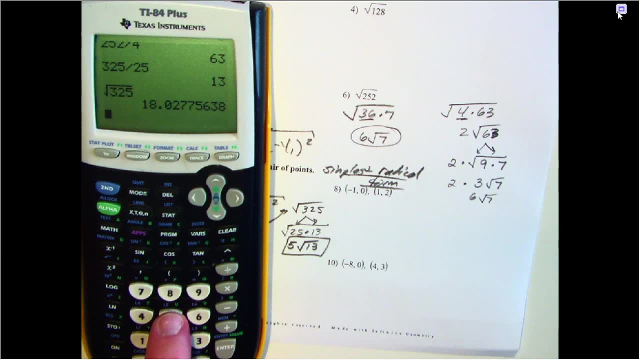 When the directions say simplest radical form and you tell me 18.5, and you tell me 18.02,, you know you've done something. I will count it wrong. But hey, you could check. did I simplify it correctly? 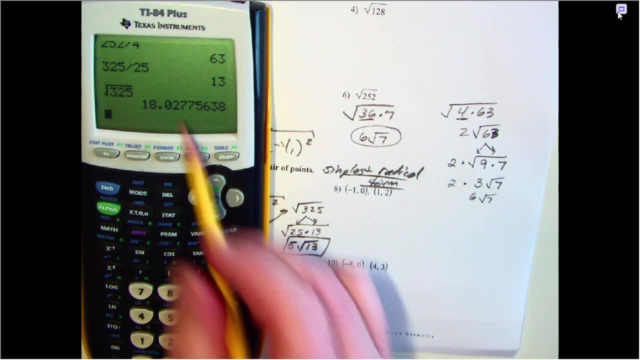 In case you're unsure, see, does this equal that 5 square root of 13,, that is 18.02.. I did simplify it correctly. I'm going to do one more of these, and then you guys will be ready to rock and roll here. 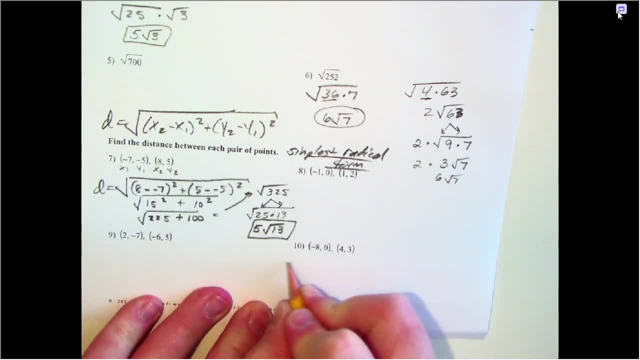 Let's do this last one down here. So the distance is going to be the square root of you. just need to subtract the Y's. In the end, it doesn't really matter what order you're going to do it. order you do these in, I could do negative eight minus four. Just to show you, did you get the same? 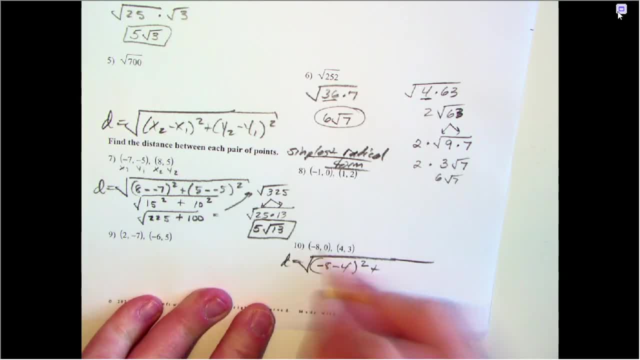 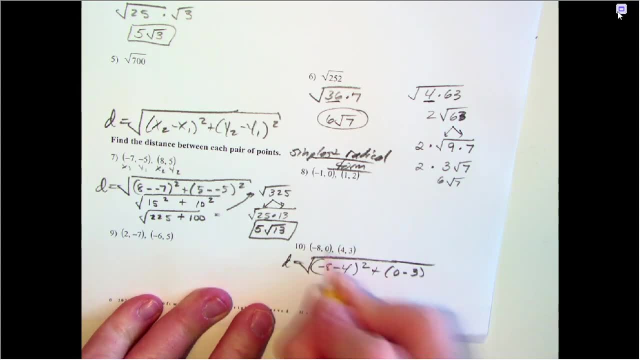 answer. It doesn't matter If you like to just go left or right, go left or right. Just be careful: This minus that, that minus that or three minus this or four minus that, it doesn't matter. Here's the reason it doesn't matter. Negative 12 squared is the same thing as a positive 12 squared. 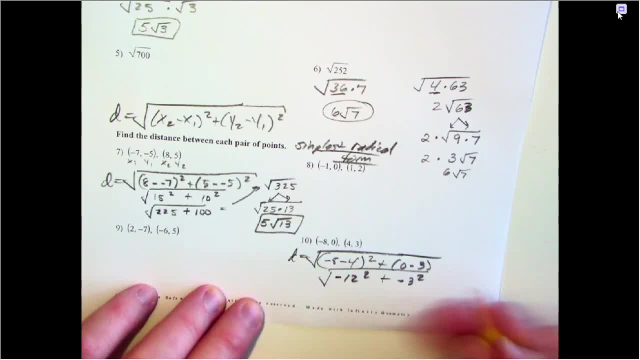 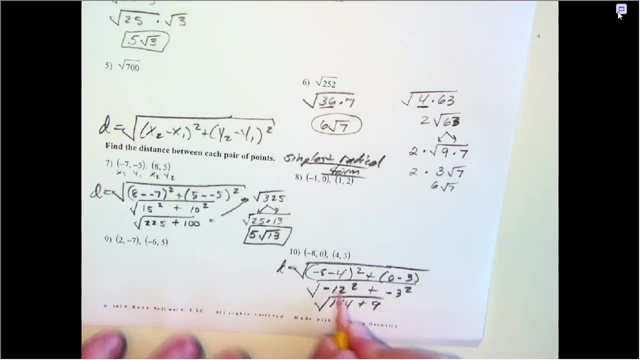 A negative three squared is the same thing as a positive three squared, So that's 144 plus nine. Where I find the most common mistakes here is students make one of these numbers negative. Keep in mind we're finding distance. It must always be positive. 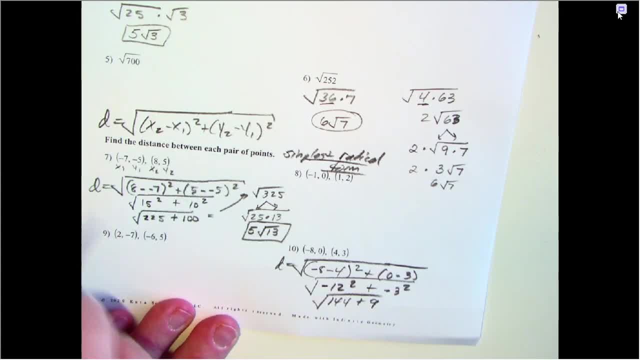 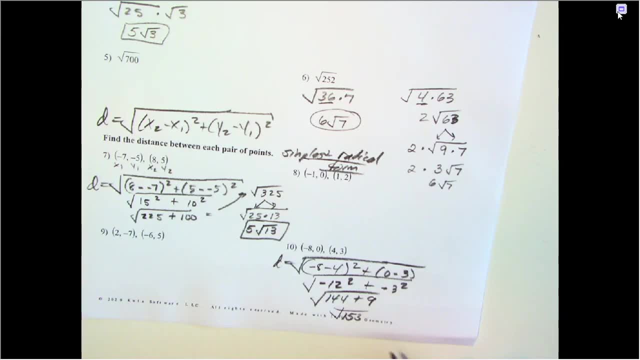 So I add those up, I get 144 plus nine. I end up with 153.. All right, So 144 plus nine, Nine is 153.. Let's see, Can that be simplified? That's what I've got to decide. 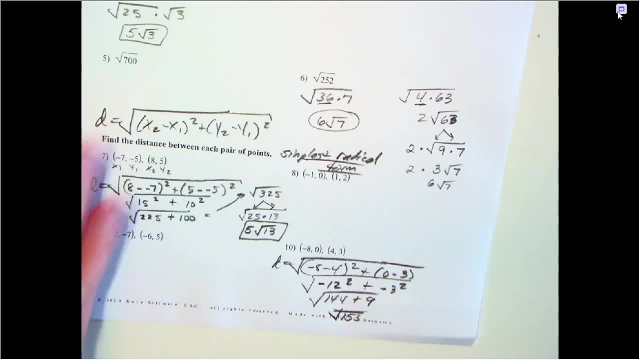 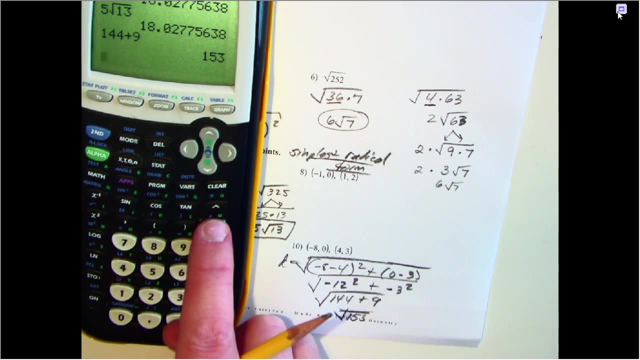 Hmm, 153.. Well, I don't know my factors of 153 besides one and 153.. So you know, I'm going to start dividing. I'm not going to divide it by two or by four, because I know that's a. 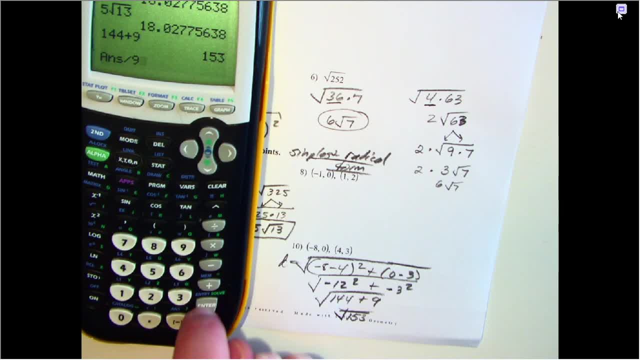 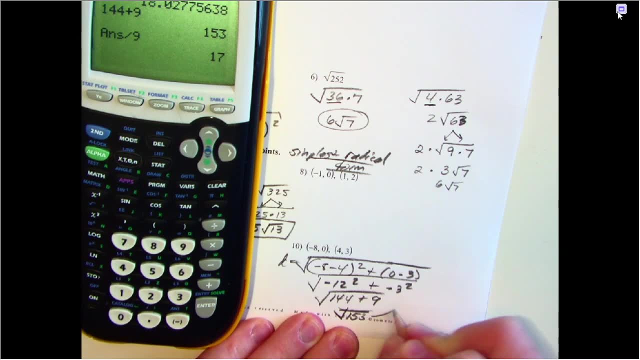 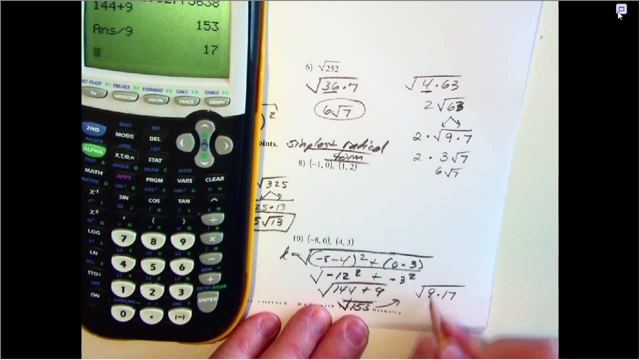 that's an even number, So let's try to divide about nine. Oh, nine goes into it 17 times. I got lucky on the very first one. So this is the same thing as the square root of nine times 17.. Nine's a perfect square. The square root of nine is three. 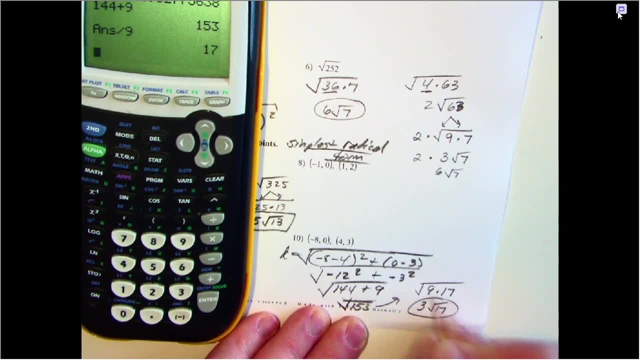 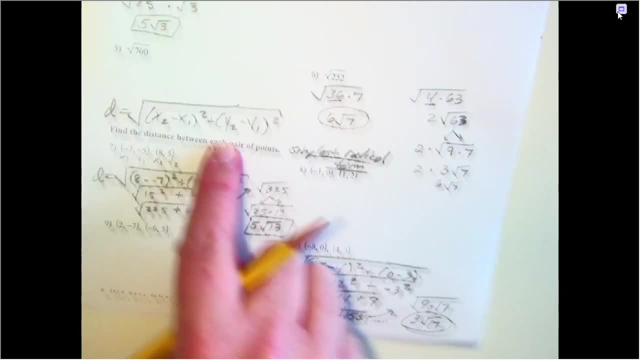 17's not perfect, so it stays underneath the radical Guys, that's how you simplify a radical. I want you to use that method. whether we're doing the distance formula, We will also use this method to leave our answer in simplest radical. 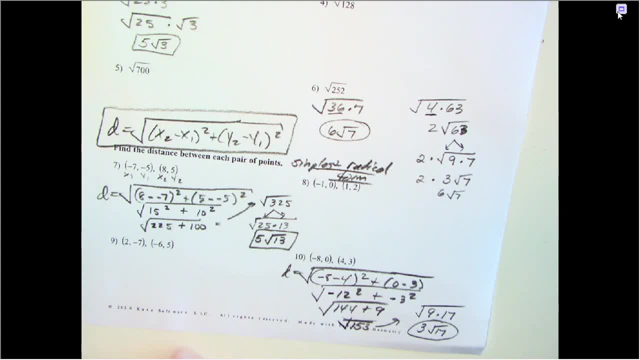 form when we work exclusively with triangles in the Pythagorean Theorem. I didn't demonstrate the Pythagorean Theorem here, but you could use Pythagorean Theorem to find the distance between two points, especially when it's on a grid. 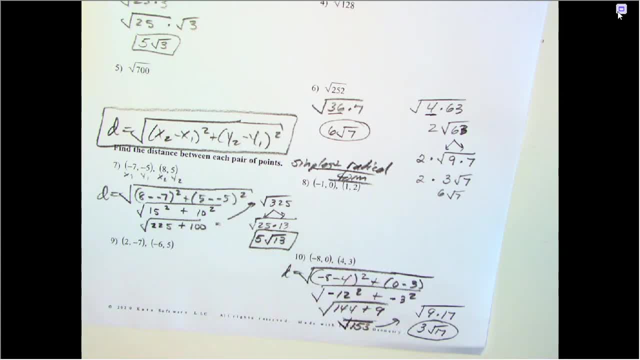 But if it's not on a grid, I would use the distance formula. I hope this- a couple examples- is helpful. Watch this video again. if you need additional help, Ask me questions in class. We'll see you later. 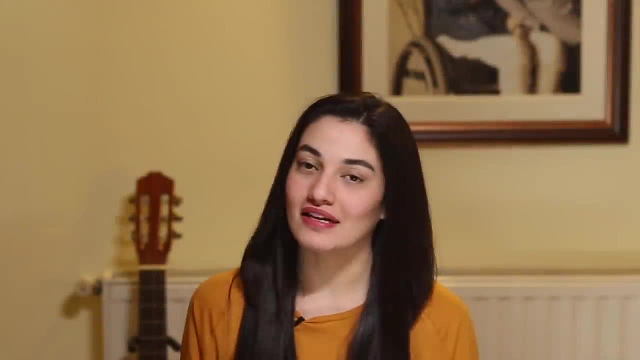 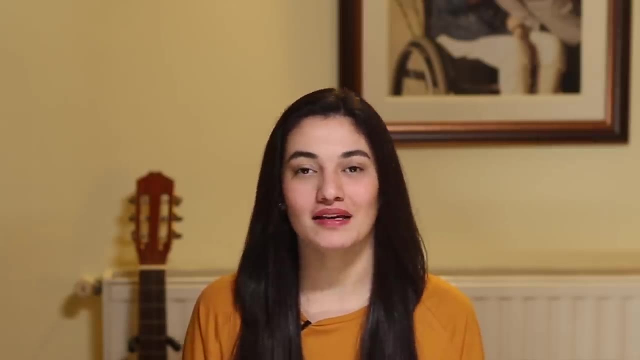 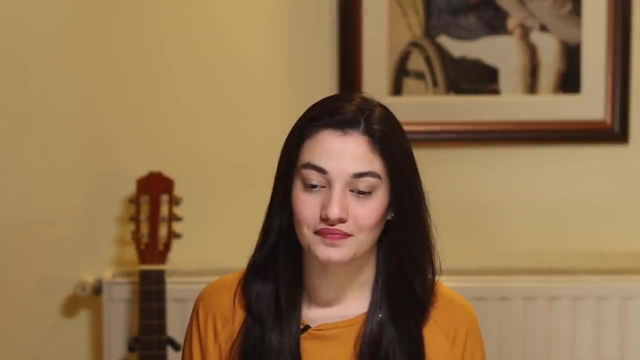 I have many life heroes and I learn so much from them every day. And one of the biggest heroes in my life is my beautiful son, Nile. He knows that his mother is different from the other mothers. His mother cannot go outside and play with him. His mother cannot go in. 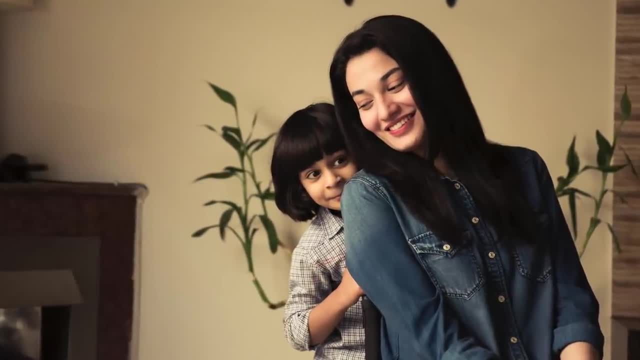 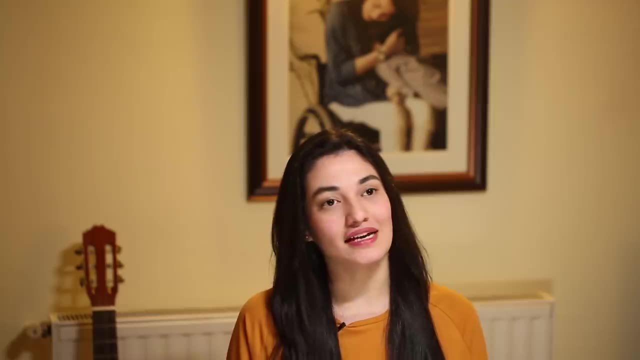 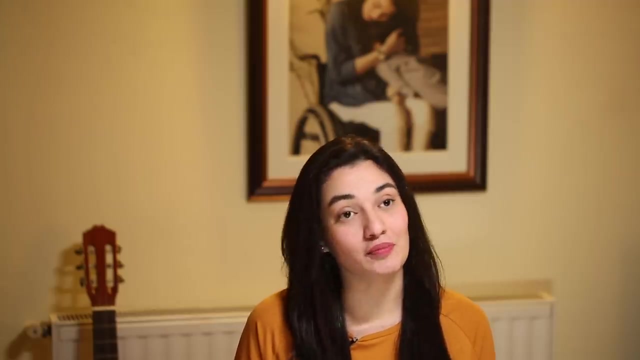 public parks with him, But how to stay calm and patient and how to keep reminding her that she is not different from the rest. I learn from him every day, and there is an incident that I would love to share. One day we were playing. you know, we decided to play.